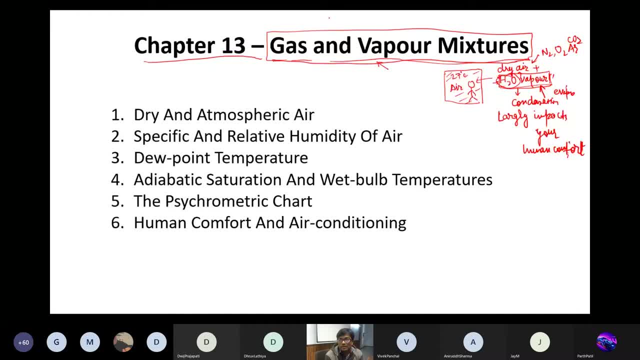 Bye, Bye, Bye, Bye. later slides that human comfort. I mean we all. I mean in for in, through the engineering. we all are here to ease our life. let's suppose you are. you don't want to walk throughout the door, throughout the road, so you invented vehicle. okay, to keep your time to, to, to save your time. 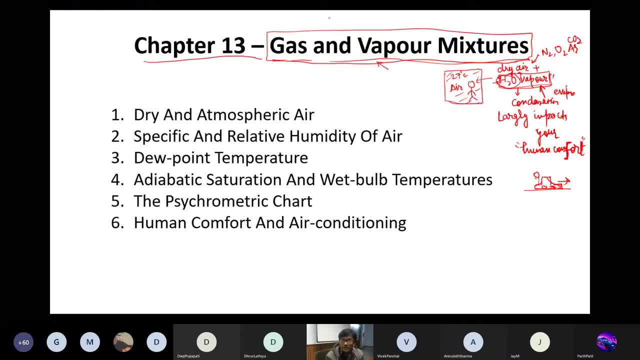 okay, so you are sitting in a nice environment, in closer, so you want things to be very nicer for you. for, in order to, let's say, you, you want things to be. temperature at, maintained at 27 degrees C, your humidity level would be certain, some, some specific humidity level you need. we don't know, don't want. 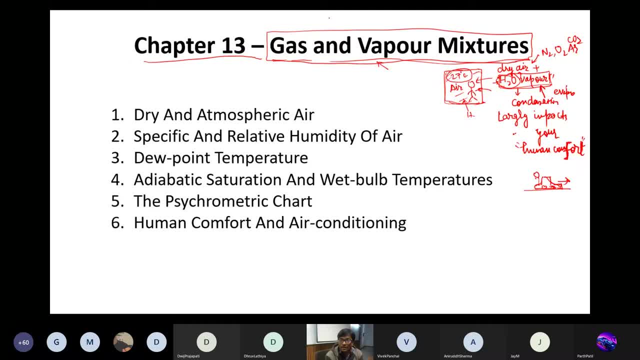 things to be at higher end or the lower end. so that's why the study of this dry and the composite of dry air, along with the water vapor that constitute the overall air, is important to study. okay, okay, in this chapter we are going to talk drier and and as atmospheric. the differences. 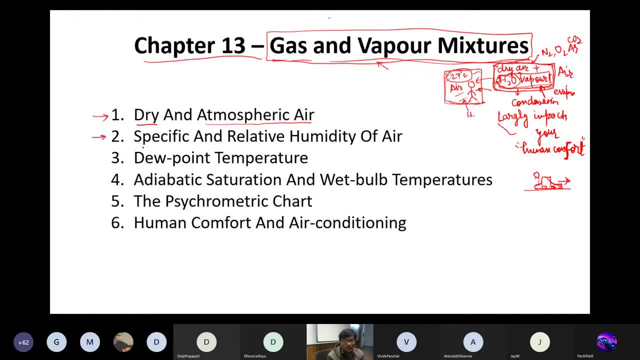 their definitions. we will introduce few keywords, such as specific humidity of air or relative and relative humidity of air. we'll also talk about dew point temperatures and what are its implications. so where you you may feel that when in the, in the hot summer, when you take out your soda cane from your 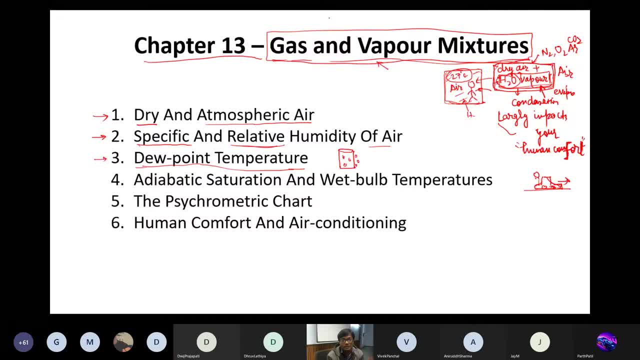 refrigerator, you will see small droplets around the kind of the, the water molecules that condense outside when the moment you X out, take out your soda, can also your. when you wake up in your in the morning, you see that the water molecules are condensed on the leaves on the leaves, okay. so this is. 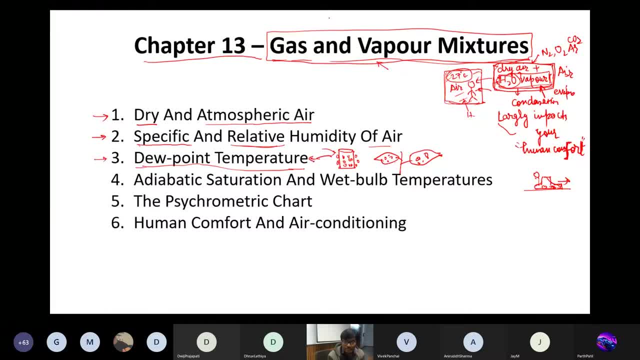 because there is something called you dew point temperature. it achieves dew point temperature and we'll talk in details some something, and next thing we are going we will talk about is adiabatic saturation temperatures, wet bed temperatures, dry bulb temperatures. the most important thing is, like our property table. we have something called. 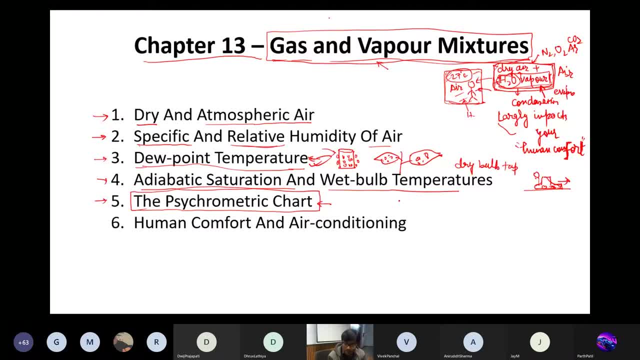 psychometric chart. your property table has a shortcoming: that it doesn't talk about the temperature of the water molecules and it doesn't talk about the humidity of water molecule in air- okay, the humidity and its essential counterparts. so that thing is missing in your property chart. so property table. so 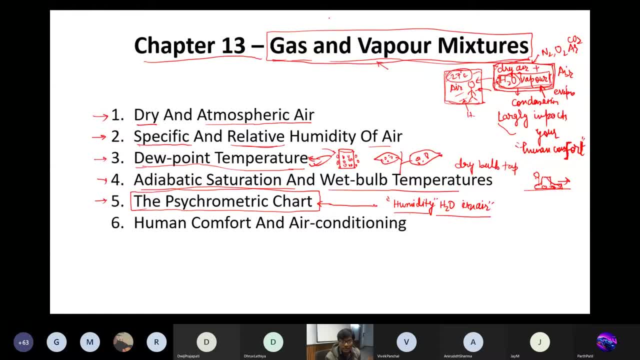 that is why we introduce something called psychometric chart, which includes all all the properties that relates these: water vapor and dry air and everything okay. lastly, we will talk about human comfort and air conditioning, and this should be our goal of this particular chapter, in order to 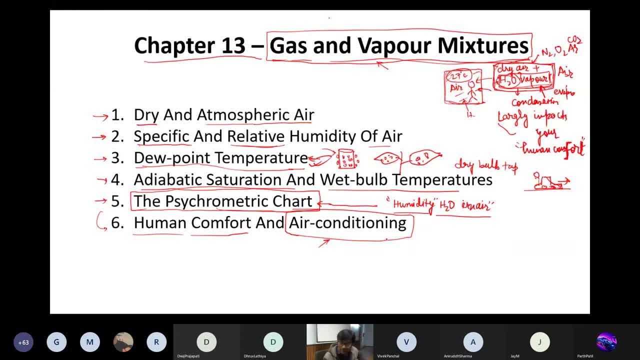 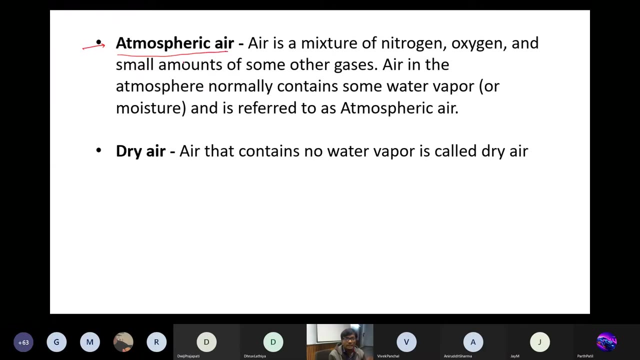 design a optimal air conditioning system, we need to know how, how the air and the humidity inside the air could be regulated in particular way. so first thing is we need to define: is the atmospheric air. the air is a mixture of nitrogen, oxygen and small amount of other gases. air in the atmosphere, the 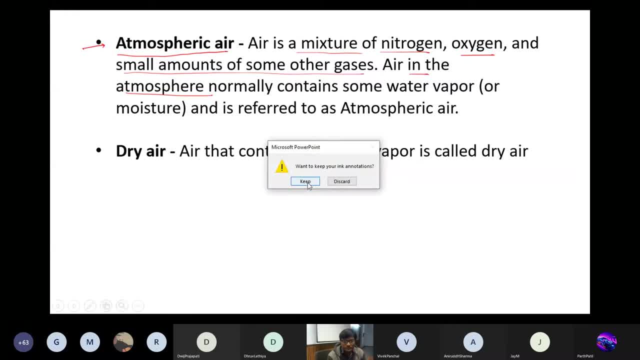 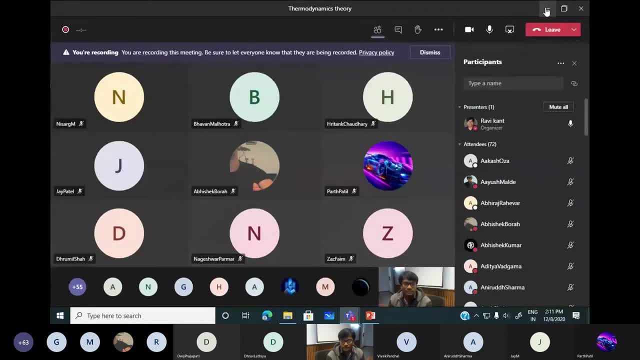 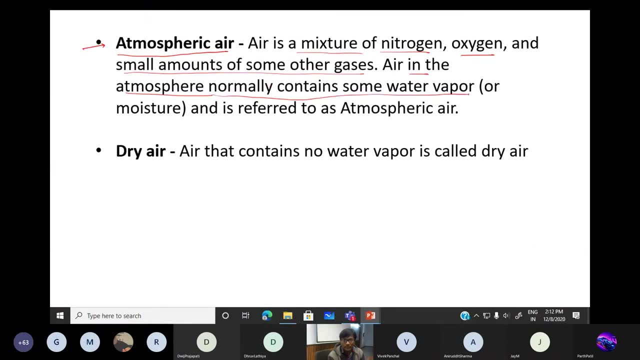 air is a mixture of nitrogen oxygen and small amount of other gases air in the atmosphere. the air in the atmosphere normally contains some water vapor as well or moisture content and the overall sense. like you have everything and two plus edge oxygen, plus o2 and other co2 plus organ plus H2O vapor, so everything. 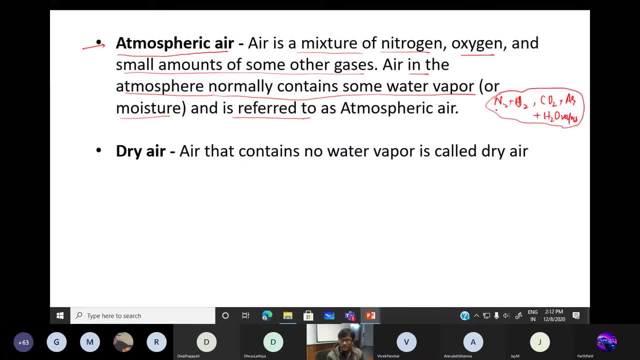 collectively the, the in certain ratio, they are in certain. so everything in certain ratio, they, they are in certain ratio, they are in certain percentage by mass. they are called atmospheric air. okay, so atmospheric air includes everything, whereas dry air is defined as the air that contains no water vapor. 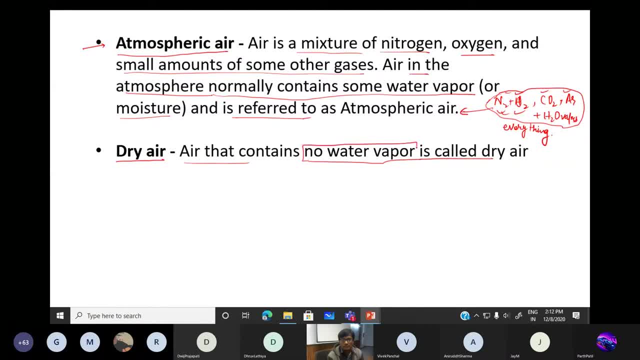 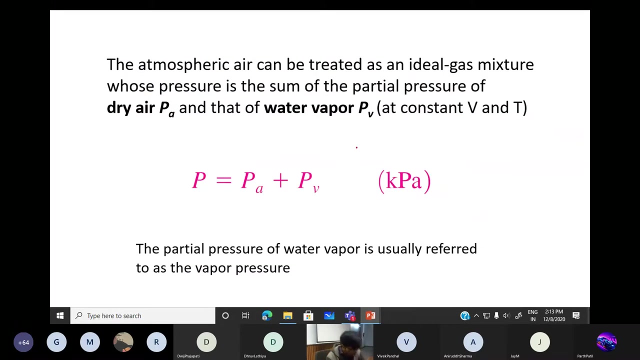 it means excluding this. so let's suppose n2 plus o2, plus co2 plus ar, we call it dry air, and plus so, except water. so we have excluded water vapor. okay, so collectivity is called atmospheric and alone it is called dry air. okay, now let's talk about certain properties that that are associated with dry air and water vapor. 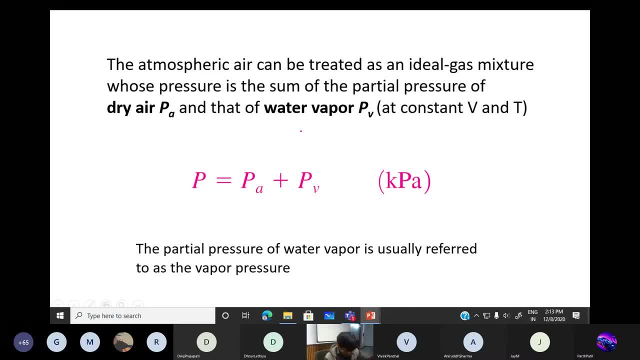 and in order to study, we need to. in order to analyze the thermodynamic characteristics of the air, we need to analyze the properties of the air. okay, so collectivity is called atmospheric and alone it is called dry air. characteristics of water and dry air. we need to ask for few properties. The atmospheric. 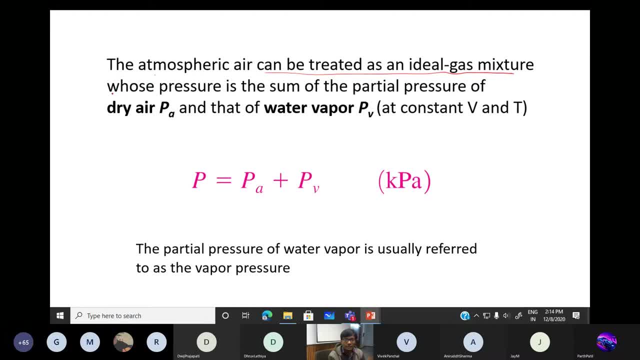 air can be treated as an ideal gas mixture. It can be, actually it can be. we have also seen that it can- if it is in proper, in certain temperature and pressure range. so temperature, pressure, lower pressure and quite high temperature, you can actually estimate your air as ideal. 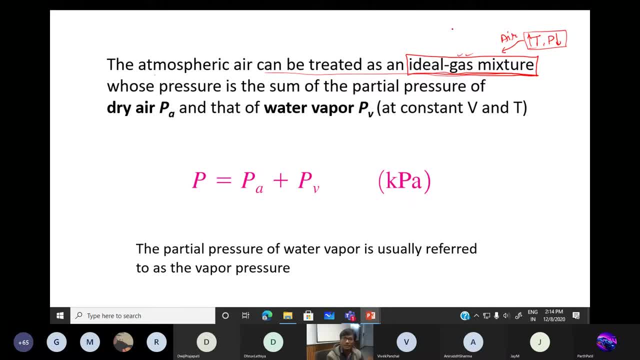 gas mixtures. You can actually apply your. what do you mean by ideal gas mixture? You can actually apply pV. small v is equal to RT. pV is equal to RT, where p is absolute pressure, specific volume, So characteristic gas constant, and absolute temperature. The atmospheric air can be treated. 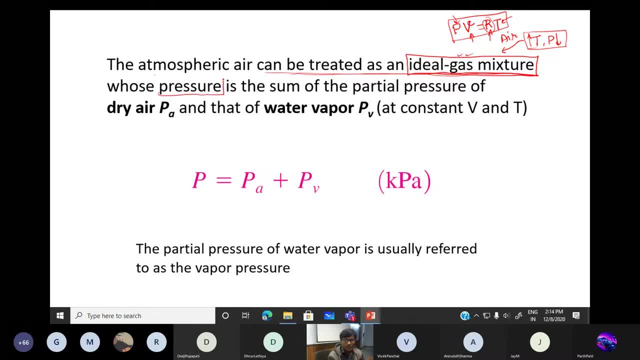 as an ideal gas mixture whose pressure? so we can actually estimate the pressure of this mixture. So pressure of mixture: mixture means mixture. it would not be a good way to write tell mixture. So total pressure. total pressure could be the sum of partial. 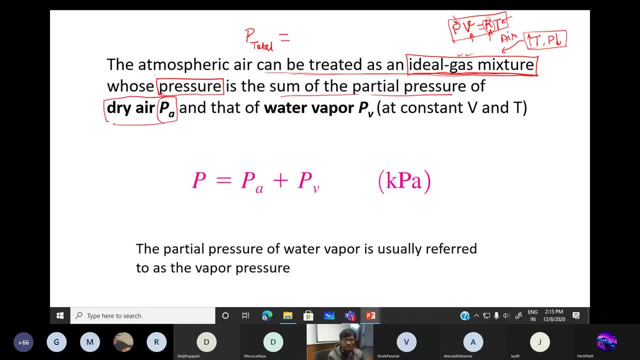 pressure of dry air, That is pA. we denote with pA subscript air. Air means dry air, not the full air, I mean not the total air. and that of water vapor pressure. that is pV. we denote it with p. 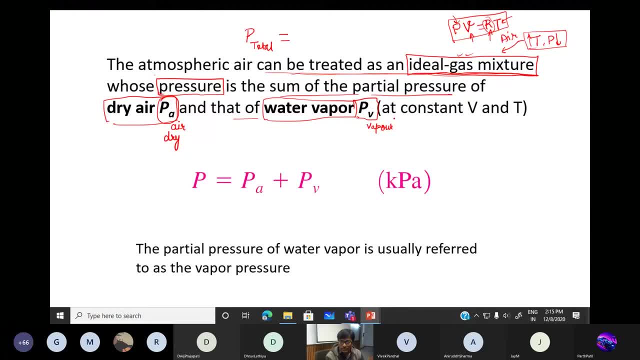 vapor, okay, And it should be at constant volume and temperature. Okay. So essentially, P total is actually the sum of partial pressure of dry air plus the water vapor, And this water vapor pressure is also called vapor pressure most often, And so this: 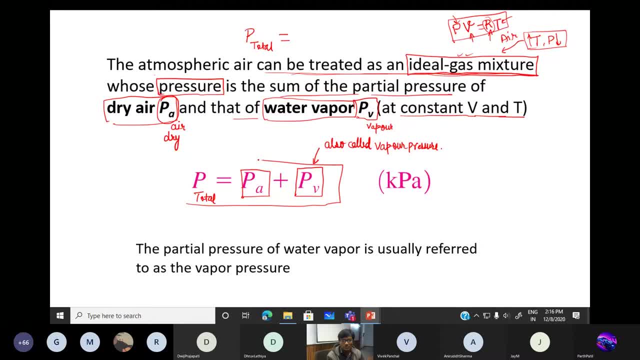 formula. I mean you should not believe this formula because I mean, how should you believe this? So there was a scientist called Dalton Dalton, Dalton's law of partial pressure. So he did an experiment and what he found out. so he 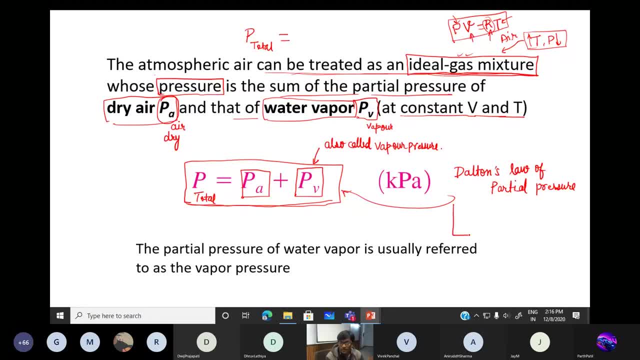 found out that he took a gas A. let us suppose gas A, and that was an ideal gas, gas A with certain volume and certain temperature, And he measured its pressure. Okay, So let us suppose this is your box and gas A was inside with certain volume. This volume? 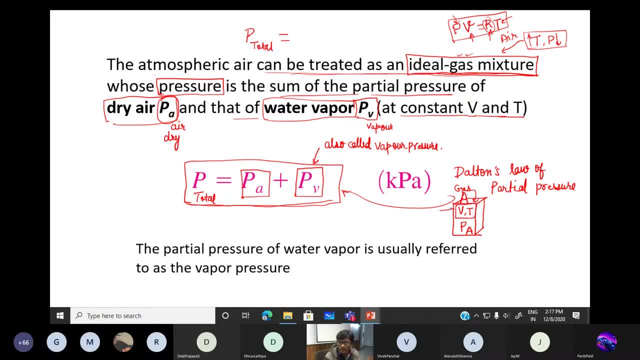 and temperature was kept constant. Okay, He took another gas at at same volume and same temperature. but here you had gas B inside it. Okay, And, and same volume and same temperature. it means the area, the volume it occupied was same and temperature it was calculated was same. 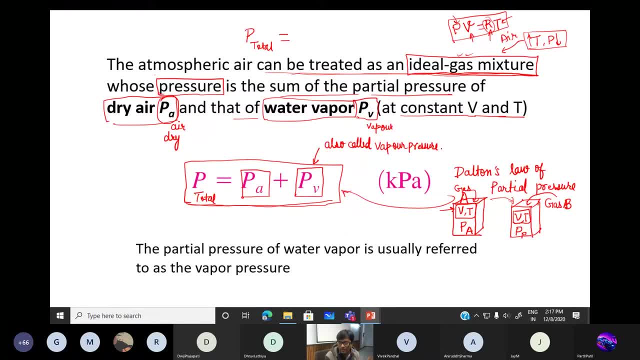 and this gas exerted a partial pressure b on that time. so what? he concluded? that when he, when he kept the gas, both the gases as in in mixture form, in the mixture form, he mixed all both the gases, mixture form of gas a and b. so this is your mixture, in same volume and temperature. so he didn't change the volume. 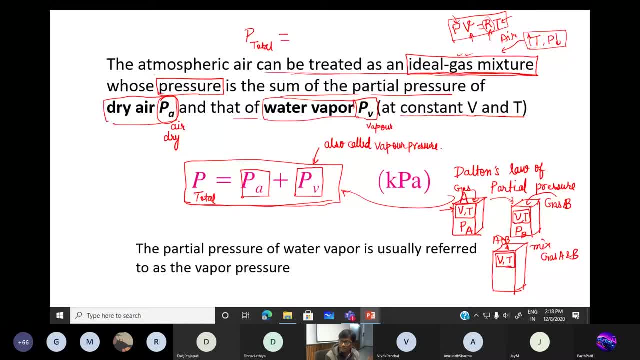 okay. so volume, he kept constant. so this is a catch: volume and temperature he kept constant. then he found out that the pressure of this mixture comes out to be the partial pressure it would have done. i mean the algebraic fabric sum of this P b and P a. From there, if we have, we can derive this expression that 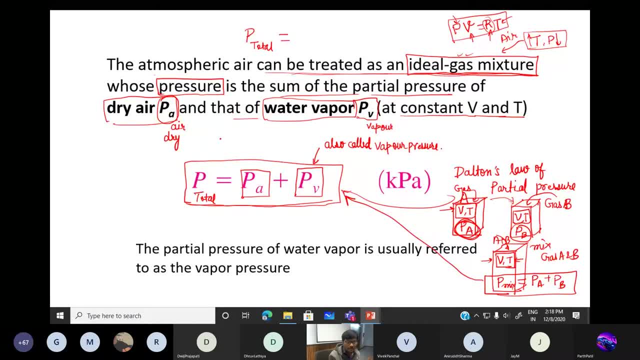 total pressure. let us suppose you have a dry air. you have, you have something A as some dry air except H 2 O, and you have a gas. B is your water vapor, H 2 O vapor in vapor form, and his pressure is P b, or this time this is P v and this is P a, and it was at constant. 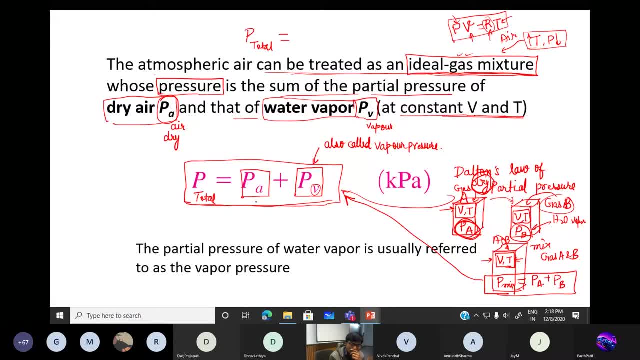 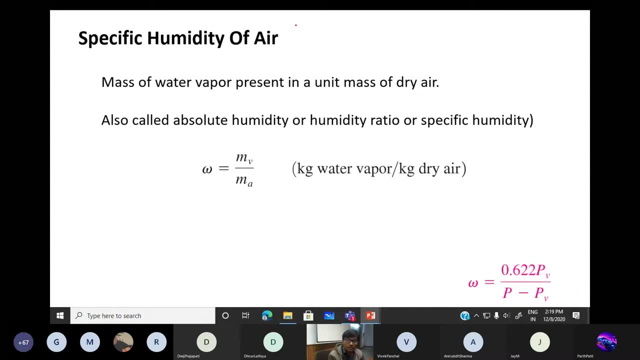 volume and temperature. it came out to be the algebraic sum of dry air vapor. ok, The partial pressure of water vapor is usually referred to as vapor pressure. also ok, There are a few variables or sorry, not variables- few properties which could signify your air. humidity means how much water vapor it contains. So there is a way to find out. 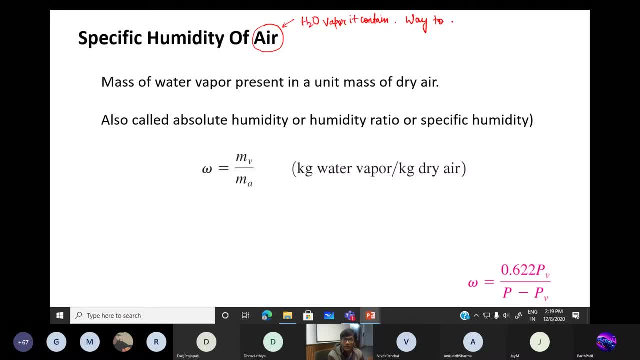 there is a way to actually define it. ok, So first, first way to define your vapor content, basically vapor content. So vapor content is specific humidity of air. we define something called specific humidity of air and it it is defined as the mass of water vapor present in unit mass of dry air. 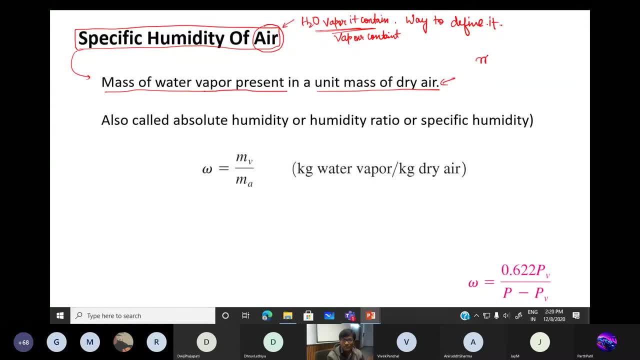 What does it mean? So you take a mass of water vapor m v- we call this v subscript- divided by mass of air. Ok, Mass of air, that is dry air and this is water vapor. H 2 O vapor mass mass. ok, this is the. 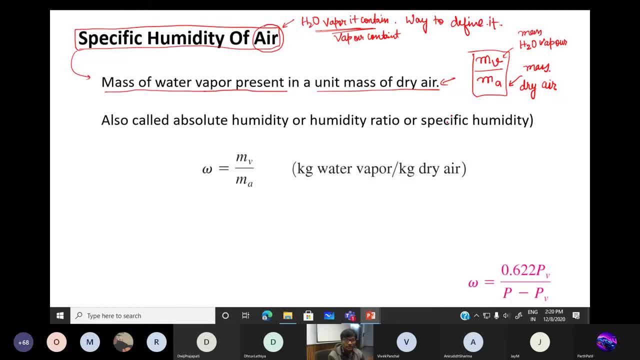 ratio and this is how you are, you can define. So it is sometimes also called absolute humidity, also called humidity ratio sometimes, or specific humidity. So most often it is, we call it specific humidity and if we generally, we define specific humidity with omega symbol, which is mass vapor by mass air. So whose ratio if this would be dimensionless? 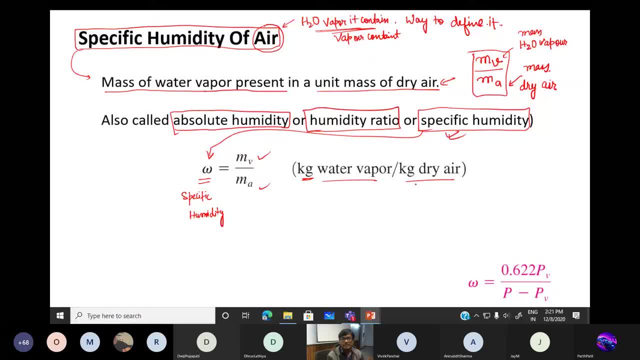 because both will be in kg s kg water vapor by kg dry air. Now, since we have already- Right, Yeah, already- estimated that my dry air is dry air, is an ideal gas, So can I apply the ideal gas law to find out what mass it could contain with respect to its pressure, volume and temperature? 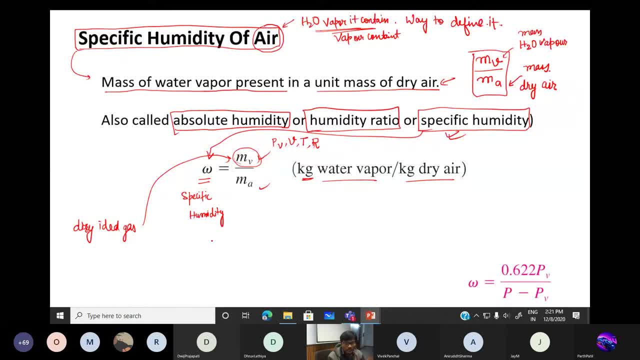 and obviously gas constants. Yes, we can do that. So we can also write omega as what would be your mass. So p small v is equal to RT. p capital V is equal to mass times, RT right capital V. So mass can be written as p capital V by. 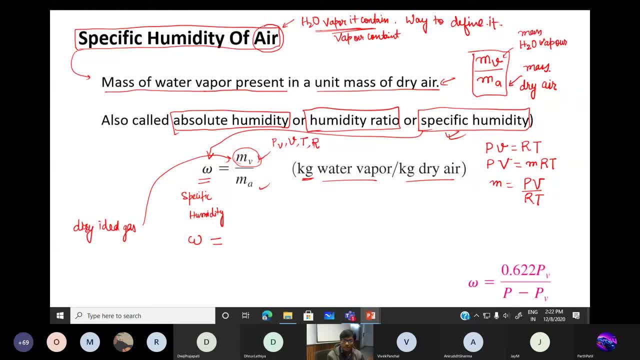 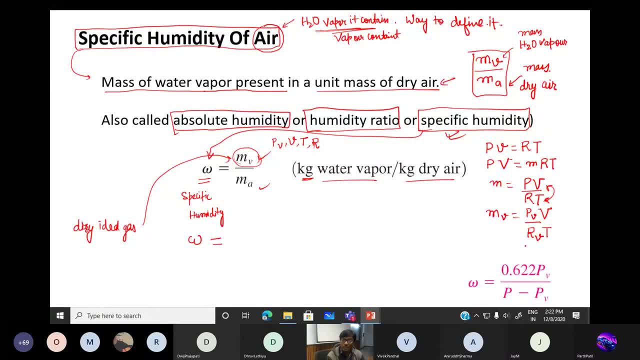 as V. So it means gas constant for your water vapor. That is the catch. Similarly mass of air. So this I will write it here. So this I will write p. small v means vapor. small v, subscript. This is subscript here. Capital V divided by R, V, T, total divided by. 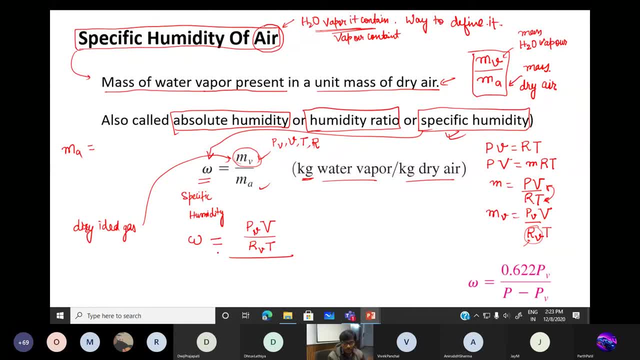 mass of air is equal to, similarly, p of dry air, total volume divided by R of air gas constant for air. So this is the total volume of air. So this is the total volume of air. So this is the total volume of air. 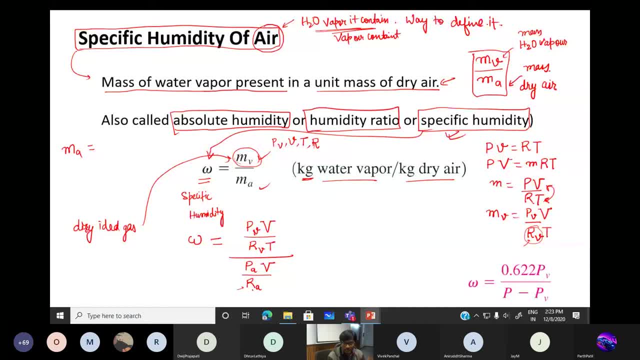 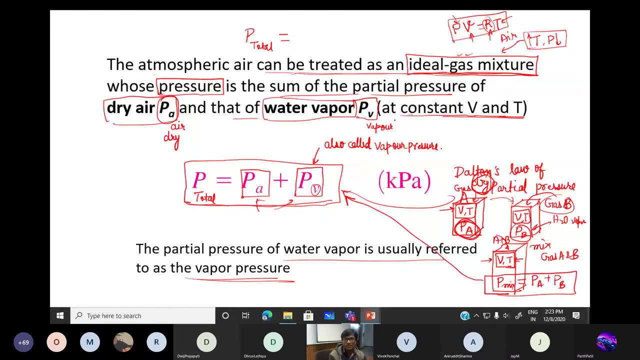 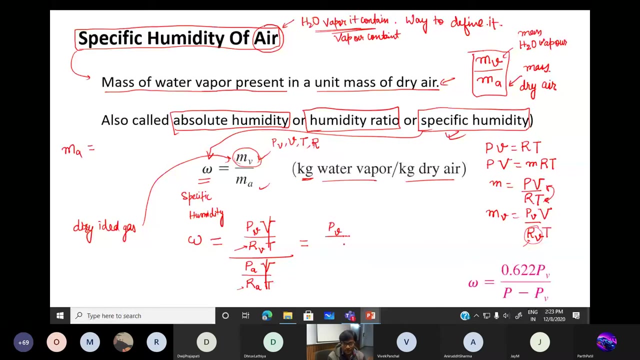 And sorry, characteristic gas constant for air, characteristic gas constant for vapor and the temperatures. So volume and temperatures are no more significant here. We can strike it out because we talk- we have already talked that we will. we will call these partial pressures at constant volumes and temperatures. So this comes out to be pV by pA R capital. 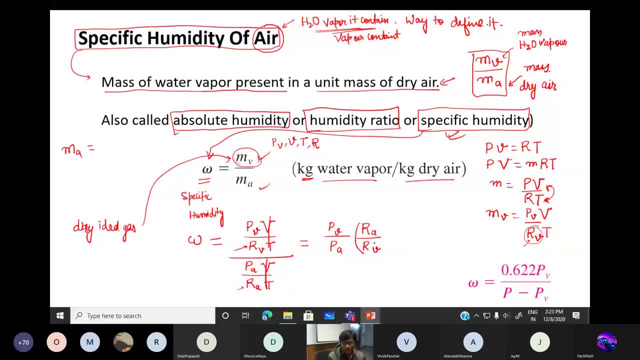 R A by R V ok. So this R A and R V people have found out this ratio of air versus experimentally they have done, they have found out and this comes out: this ratio comes out to be 0.622.. So here your omega: specific humidity of your air. total air ok can be written as 0.622, partial. 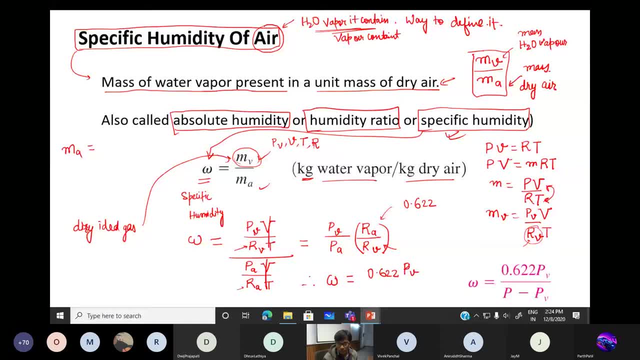 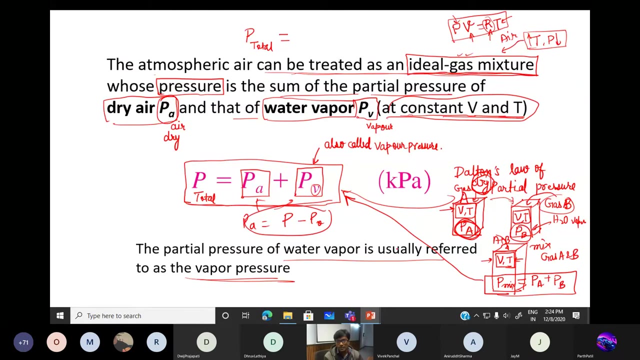 pressure of vapor. ok, partial pressure means alone, divided by partial pressure of dry air. this is the ok. One more thing: we can also write this P A as P A as total pressure of air minus P V, right, So we can substitute it here and we can get. 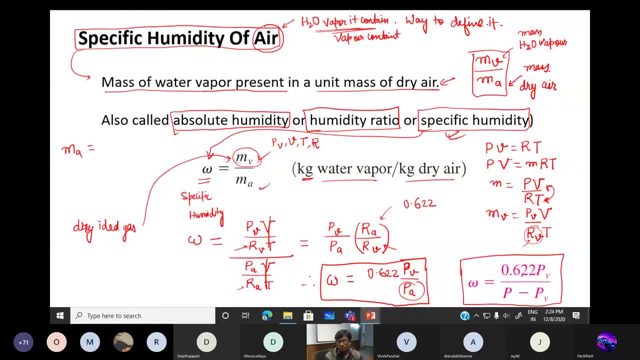 this formula right in any problem. so far, ok, but so far I was happy that I was happy that I was happy that I was able to write this formula. So now I am going to write this: I can actually know how much water vapor was present in the air with this particular 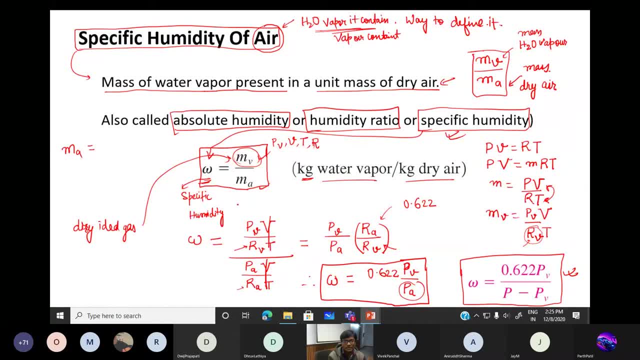 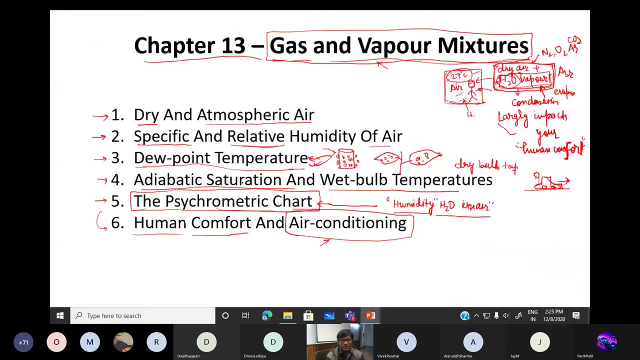 ratio. if I had this ratio- specific humidity ratio- I can actually, I am happy, but I am not that happy, the reason being this particular mass of vapor. So I could Think of another variable, I could think of Another, another way to. 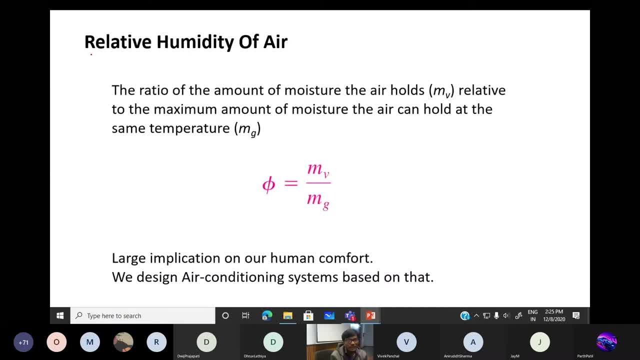 To think about it. So there comes something called relative humidity of air. ok, and now why this relative humidity has come? because I know that the moisture content air can hold right now is MV, but it can actually contain More moisture or it can also contain maximum amount of moisture air it can hold at same at that particular temperature. 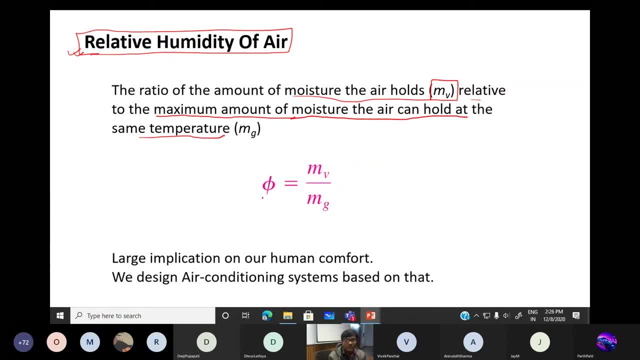 It means there is another way to define humidity of air: as relative humidity, As mass of the water vapor that currently it possesses, your, your, your, your total air currently possesses, Your, Your total air Currently possesses, divided by the mass of- I am really sorry- mass of vapor it currently possesses. 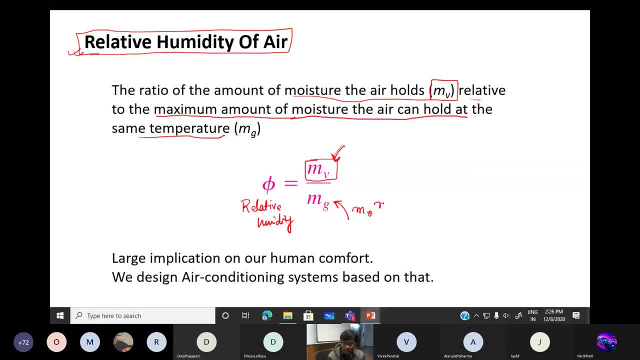 and mass of vapor. it may contain- sorry mass, sorry, not may contain mass of vapor. it maximally maximum, maximum mass of vapor it can contain at that temperature and we will come back to this once we understand something called saturation or saturated air and we will come back it to it, but just for the glimpse. you, you should know that I mean there is another. 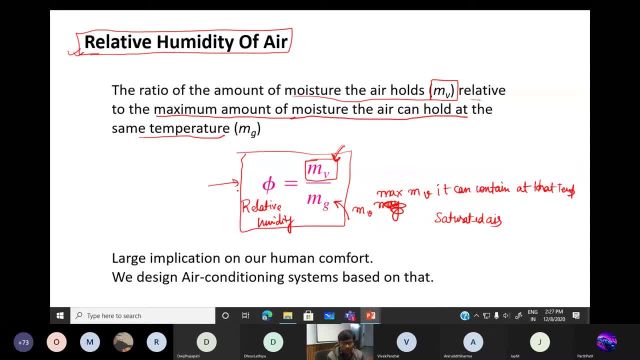 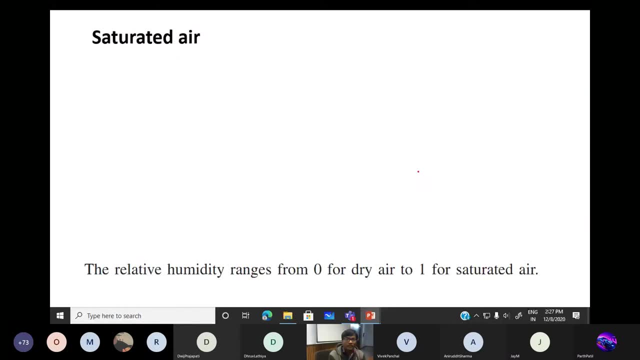 way to define your uh humidic humidity, uh humidity characteristics or humidity humidity parameters. you can also define in terms of relative humidity in this manner, and we'll see why it is important once we understand the saturated air condition. so let me come back to this particular concept called air. 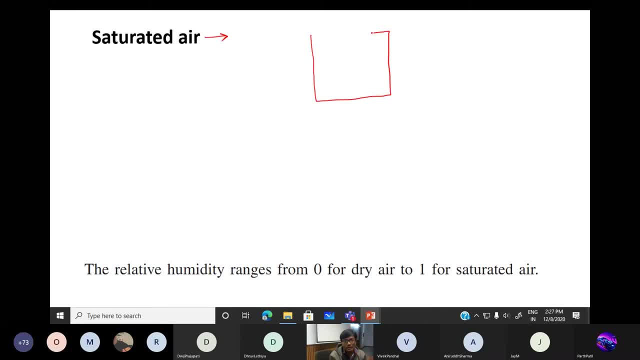 saturated air. so let me see, let me tell you one experiment I am doing, I will, I may, I want, may want to do is this: let's suppose I take one kg of dry air. so dry air does not contain uh, h2o vapor, it doesn't contain currently. 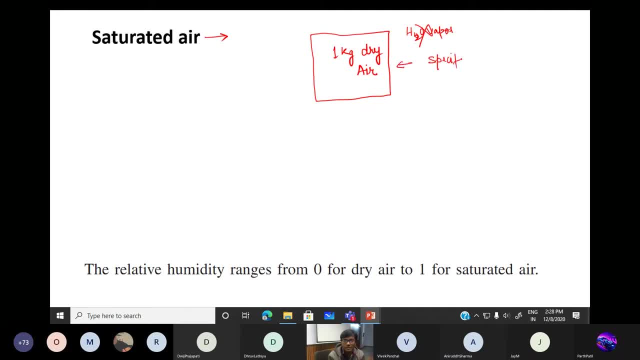 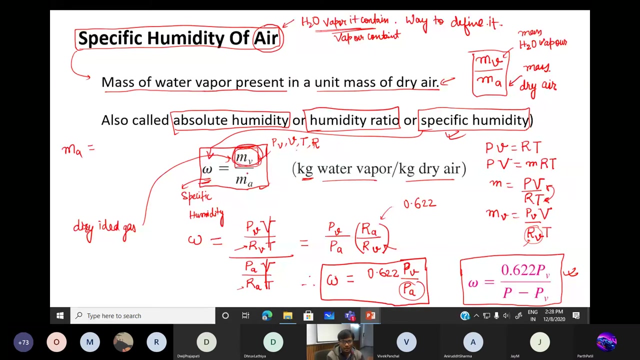 so what is the specific humidity of this specific humidity currently? humidity: can somebody tell what is the specific humidity currently? it contains quickly what I told: specific humidity is the mass of vapor. that is zero. so specific humidity is zero currently for dry air. so mass of vapor, mass of dry air. so 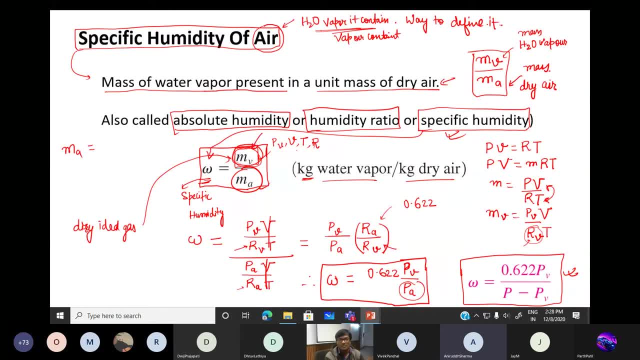 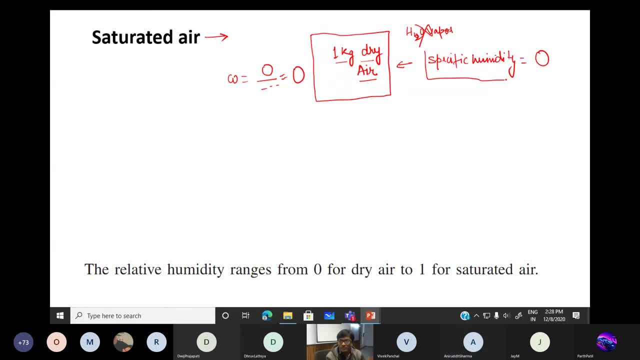 mass of vapor is zero. sir, humidity: fine, fine, fine, just, but I, I wanted, I wanted a specific answer, specific, specific answer. specific humidity of dry air would be zero, okay, okay, uh. so in this class i, i, i encourage you guys to speak in english because two of our students are not able to understand, so they may uh feel. 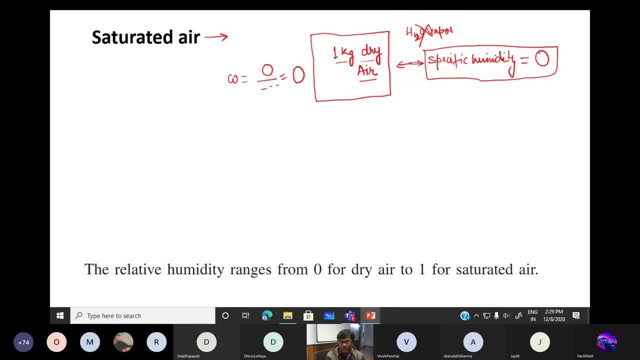 outcasted when we speak other language. so we will try, in this particular class, we will try to speak in english only, even from your side. also because they, they should feel uh as, uh as a whole. i mean they should not feel outcasted, that is what. okay, fine, but in uh, other batches, in d2d batches, uh, i. 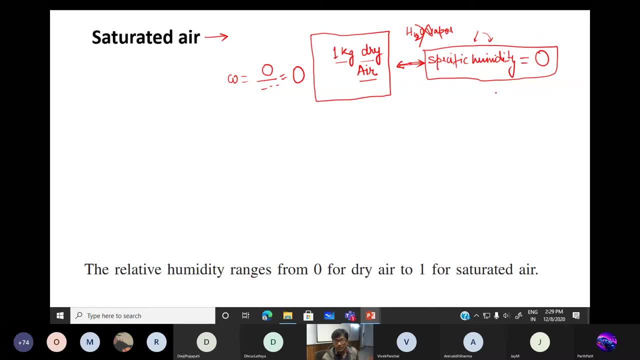 some, some. sometimes i switch because there are no non-hindi speaking students there. okay so, but here we should stick to english all the time. okay, fine, okay, uh, where were we? okay, so we have. uh. initially, we had, uh, zero specific humidity of this dryer. there were no water vapor uh contained in this particular air. now, what i do? i started bombarding. 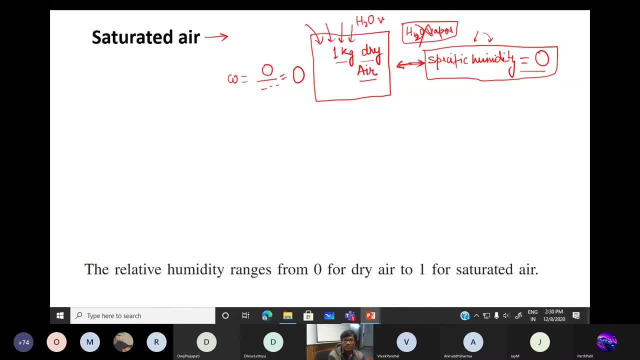 uh, water vapor into it slowly. okay, what will happen? the specific humidity will keep on rising, it will keep on rising, keep, it will keep on rising till a point, till a point it cannot hold any more water vapor. okay, okay, so till this point, till this point, you will have certain water vapor that is homogeneously mixed. 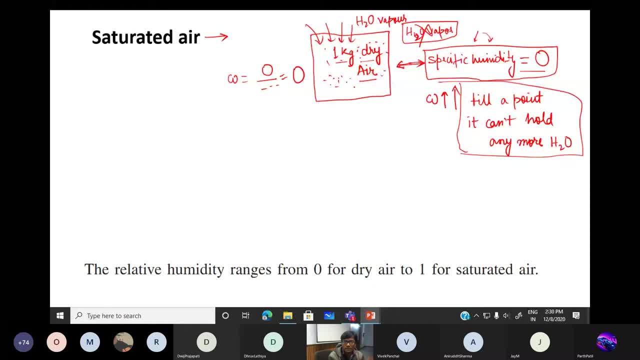 okay, certain amount of water vapor, let's suppose 0.001 kg of water vapor. i have mixed and i see that after that, uh, it cannot hold any more. water vapor, vapor, vapor, okay, water vapor. and the moment i mix it in the second亞, the next molecule of zosta vapor, now i see water droplets condensing. okay, now this condition is called about to condense. 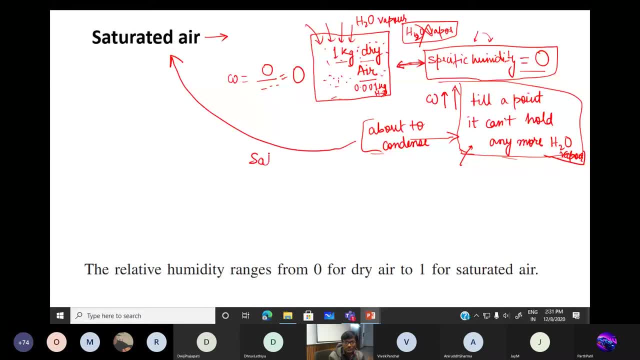 okay, and this particular condition is also called: the water has been a sorry, the air has been saturated, so this condition is called saturated air. such as saturated air means what saturated air mode? it is the basis for fat, country water vapor itself and some other state of the medical system, such as forน. 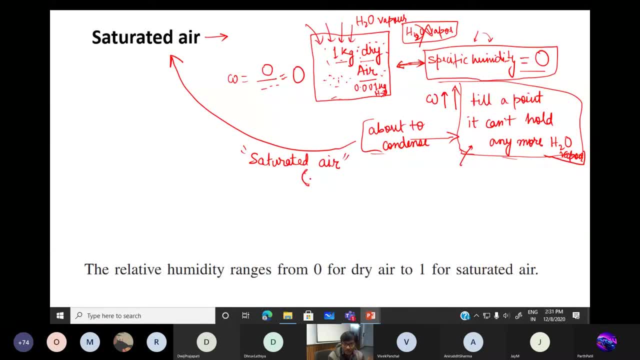 saturated, that the here the thing is hidden- is saturated with water vapor. agree, so this thing is hidden, actually, but it's not explicitly written. but we often call it saturated air. this, this condition is now: your air has been saturated. it cannot contain any more h2o water. 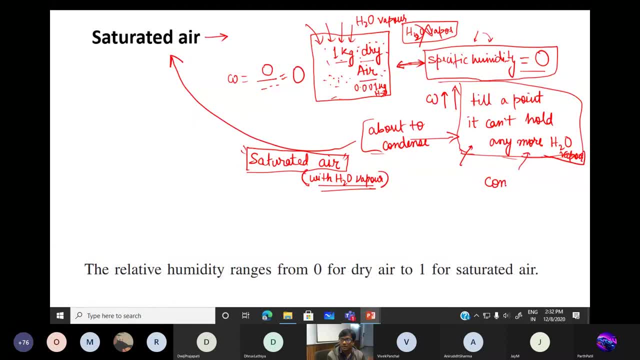 vapor. once you add more, it will condense. it will be condensed in the droplet forms. okay now this experiment i did at particular temperature. temperature, let's suppose t1. now what i do. i did same experiment at temperature t2. i started with one kilogram of air. 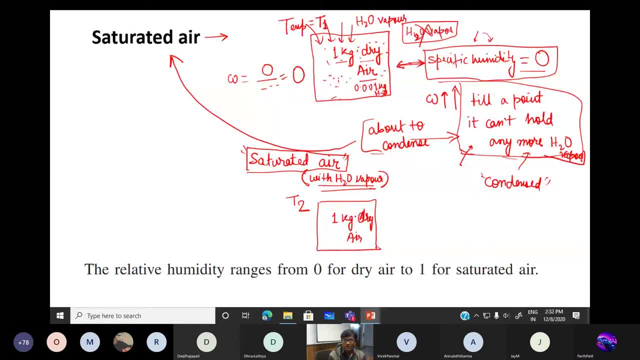 dry and i started with zero, zero, mega, but at t2. and now i bombarded it with vapors and i see that it contains- let's suppose t2 is higher than t1. now i i see that it contains 0.002 kgs. wow, now it contains. 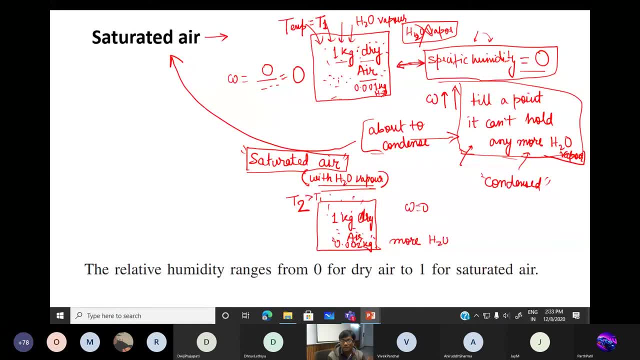 more, more, more more water vapor as compared to my lesser temperature. okay, now we did the experiment, so what i conclude? okay, uh, finally, i mean fine, if you increase the temperature, you see that it is your, uh, your saturation, i mean saturation of air, is also dependent upon your temperature. 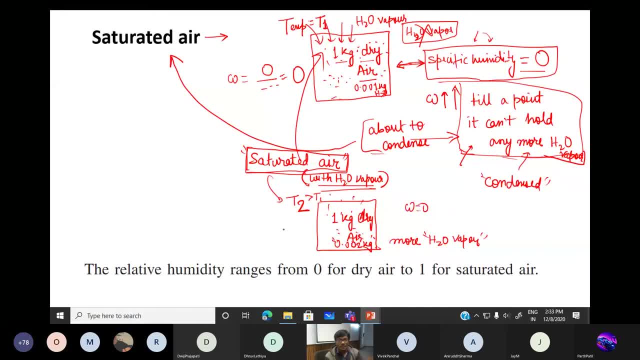 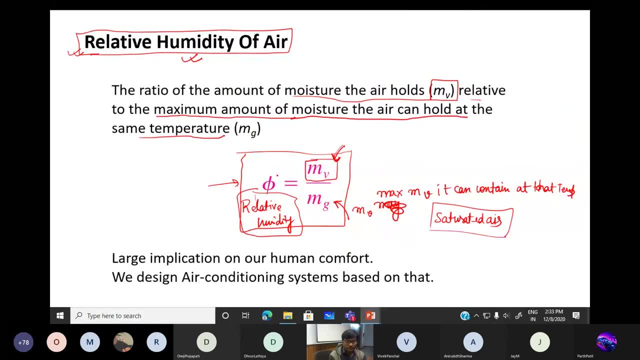 that is what we concluded. okay, now the we now we define relative humidity of air. okay, once you understand this, let me uh come back to this particular thing and let me re-read again. the ratio of amount of moisture air holds currently relative to the maximum amount of moisture the air can hold at the same temperature. 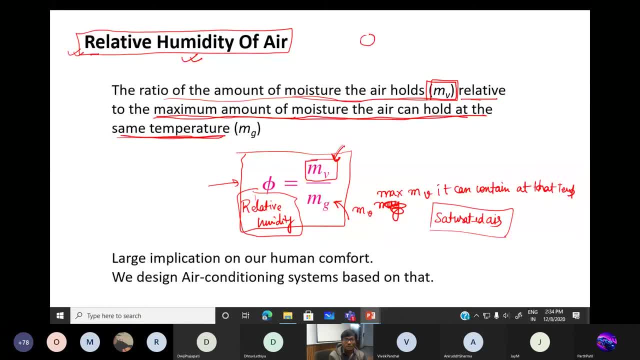 and then at the same time gets sub Mana and psi signify mountain's Great, whatever you call something. both J and I will got into that. what I have to do is: so let's just refer to the loss Z del V, by which 1 v- honestly I might be saying Z, let's. 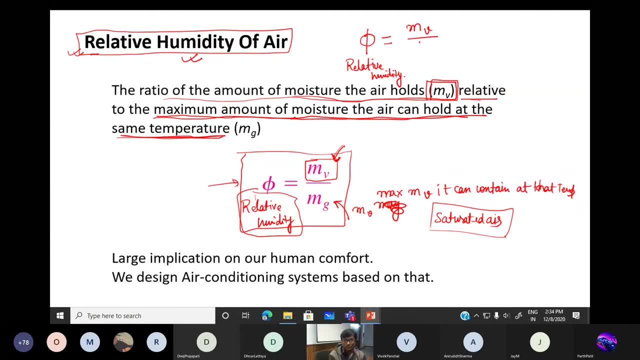 move on. so we got this concise looks'm sorry we got, hmm, anything else that I tried just because we cannot manually talk and we cannot talk right, because when you realize what kind of weight has been opened, the volume will not are generated for it. so but we have identified. 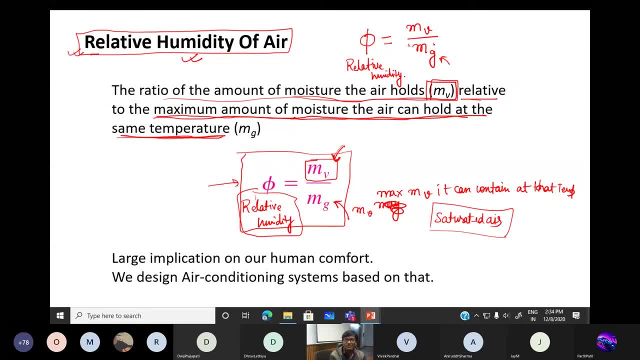 it as few in 15 minutes. do you D it, subscript this. there is a catch. So this is this subscript is for vapor, So you remember. ok, let me go back, go, not go back. let me write one more step over here. So mass of vapor. 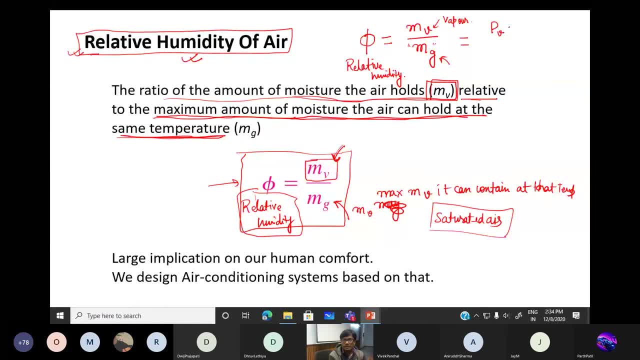 can I? can I write p small v capital V volume divided by r, v times t, divided by this mg, I can write p g. let me write this p g once then. then I will. I will tell you why. why. what is the reason? this r, g and t. ok, Now what is r v and r g? 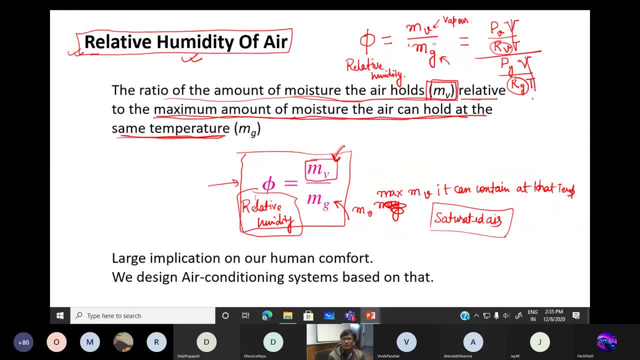 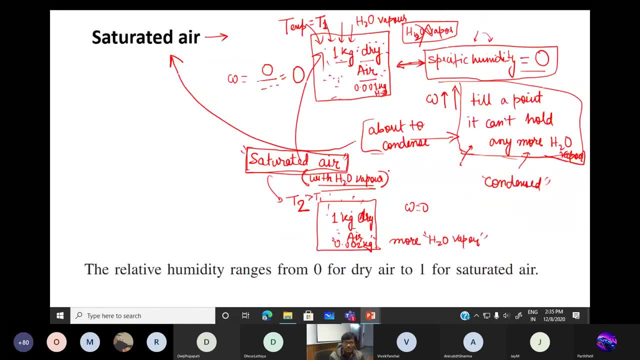 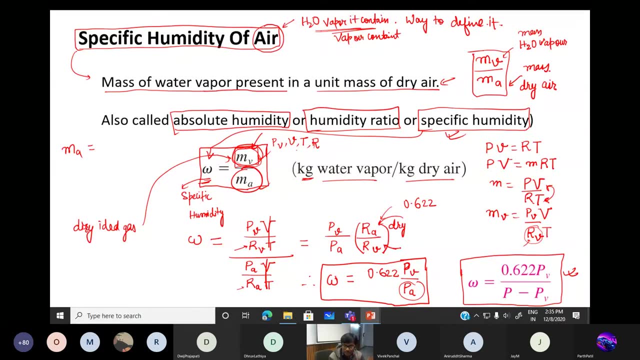 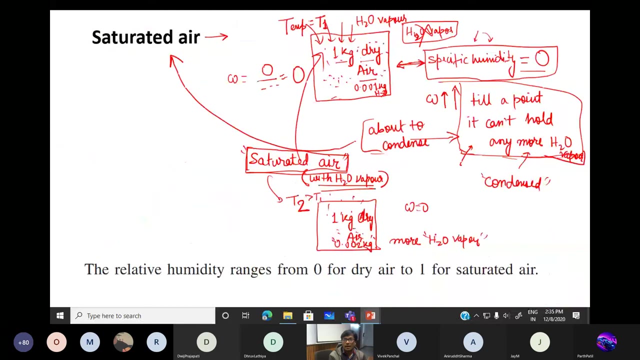 So v? t cancels out. ok, What about r v and r g? Can somebody comment? So this here in back side r a, this is: this was dry air characteristic gas constant. and this is your h 2 o vapor characteristic gas constant. and here this is r v, this is characteristic gas constant. 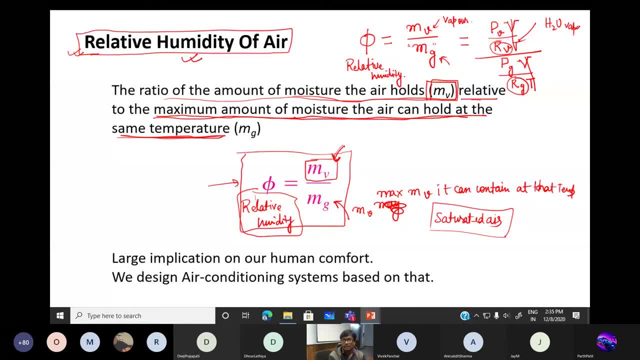 for h 2 o. and what about what? h 2 o vapor? and what about this r g? This is again for h 2 o, right? So both are same actually. So we cancel this because we are considering both the vapors: vapor, vapor contents. 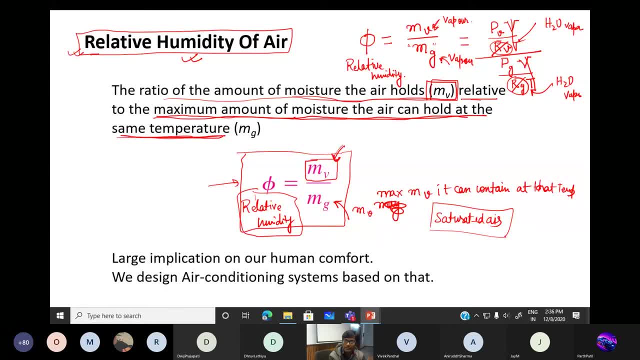 right vapor content it is holding right now vapor content it could hold at that temperature, at certain temperature, ok, So obviously I am talking about vapors only. So the both gas constants cancel out, v cancels out. So this, this thing I can write away. So this thing tell me, I can write, p, v divided. 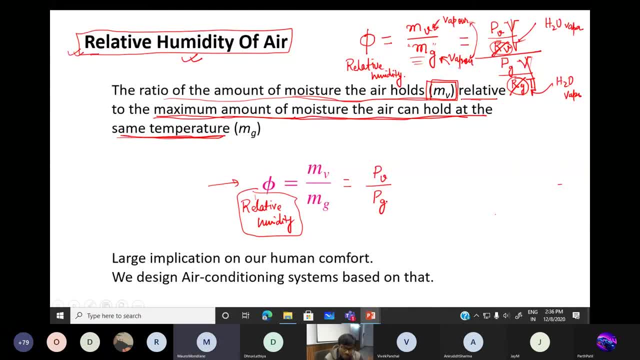 by p g. yes, tell me. Can you please just we explain about r v and r g, which one the part we so? So please tell me. Yes, Ok, So p g and p g are the same. Yes, So p g and p g are the. 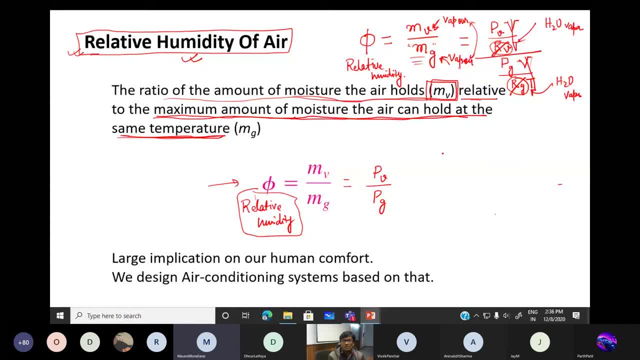 was explaining about rv, rv and rg. rv, rv and rg. okay, okay, let me go back again, so let me write it over here. these things come write it here. so this is mv by mg. so this is the some mass of of what mass? h2o vapor mass. mg is also h2o vapor mass, but that is the different. 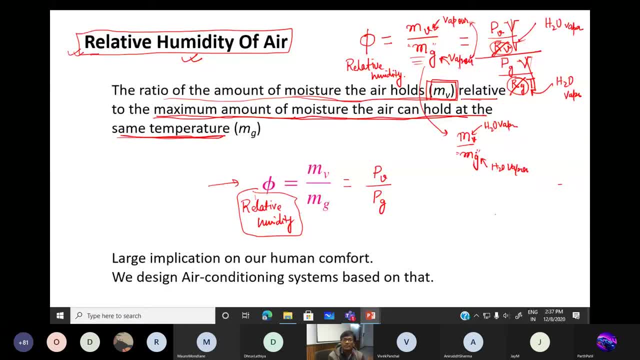 case that we are talking about this mass at this mass would be the maximum mass that it can contain, but the the catch point is both the things i am referring to the same water vapor, so their characteristic gas, constant rv and rg would be same. basically, i am referring to the same thing. 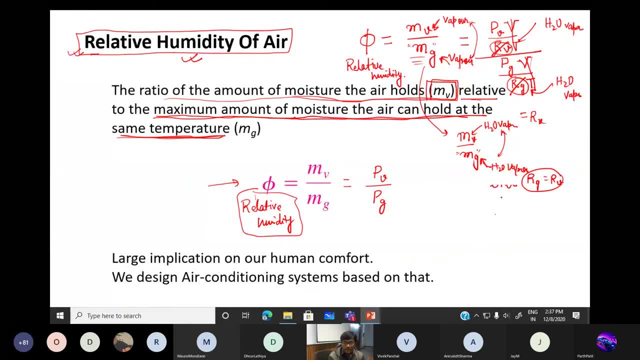 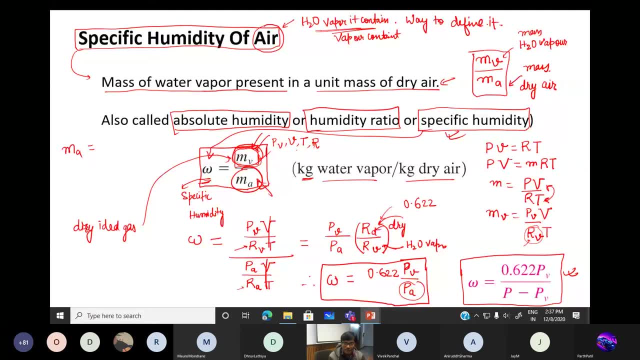 same material, same substance, but here, as compared to here, we are talking about mass of vapor and mass of gas, dry air. both are different substance. so this dry air is different and mass of vapor is different. that is why we took the ratio and this, this ratio, comes, comes out to be 0.66 by experiments. 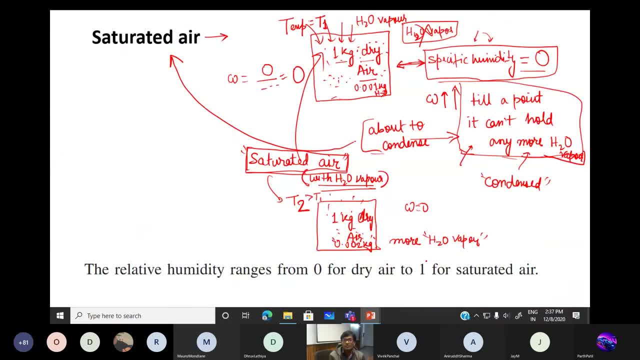 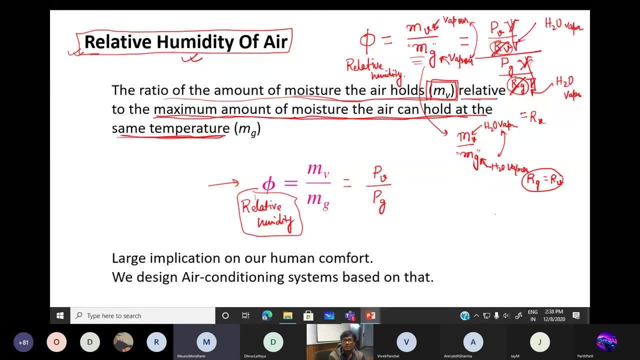 but here i am referring to the same substance, right? so that is why i cancelled rv and rg. so v and t is obviously. it was cancelled because we are considering things to be at same temperature, same volume. so so we are left with the pressure, partial pressures of vapor and partial pressure. 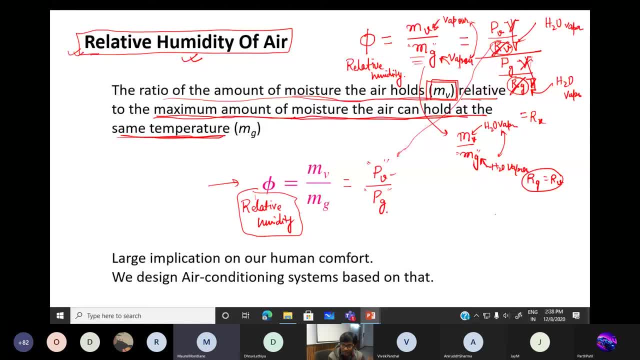 of the vapor, when, when it contains the maximum vapor. right, yes, sir, exactly. so now the point i am making here. now we will connect it with our, the usual dome. okay, so let's suppose this is your p, this is your v, and i am talking about the temperature. 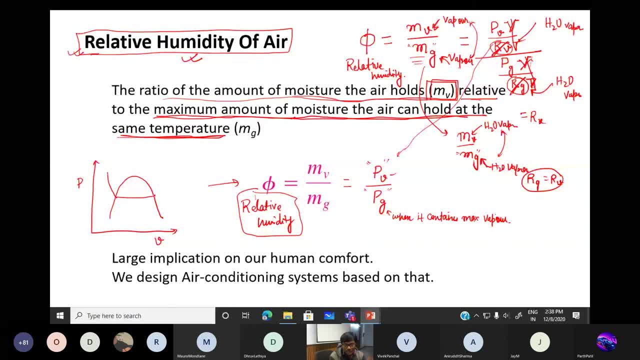 so this is your constant temperature lines, right? okay, now, at this constant temperature, this what could be the partial pressure at when it contains the maximum vapor, or it when it was about to condense? what was that point? it was this point. remember, this was your saturated vapor. so that is why i am so. 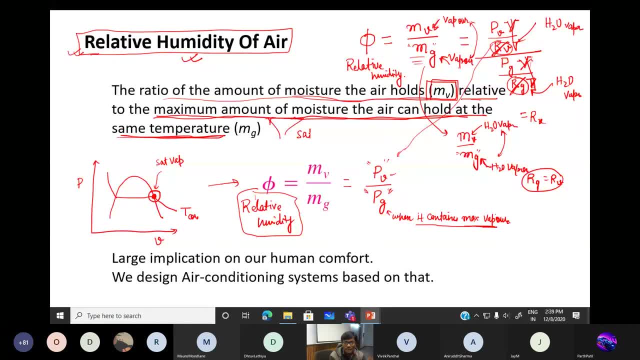 saturated means maximum amount of moisture means saturated condition. saturated condition- okay. and saturated condition means you were talking about no, not here, not here. you have to keep reached over here and then you will see. i mean, this is the point where it contains. so this is what is this point? this is your p sat. 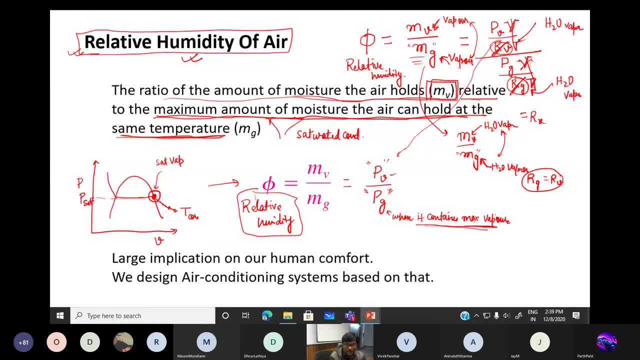 right here. it has some p, okay, but in in some p, i mean in some p you have okay, fine, this vapor pressure was there, but but there will be an hypothetical condition where the pressure reaches to saturation pressure, then only it contains maximum vapor. so i can i replace this pgy? 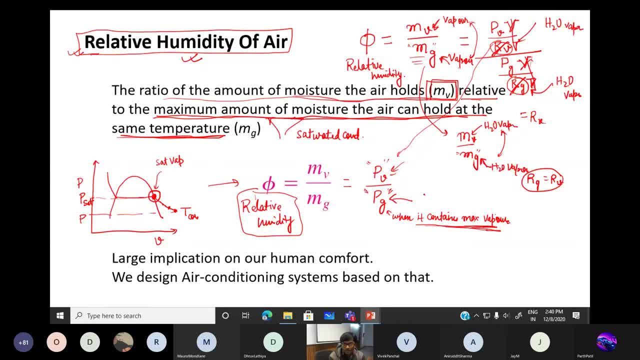 by p sat at that temperature. yes, i can do that. so this is the final formula which i am referring to and you can actually connect it with your usual thermodynamic analysis for two-phase systems. right, remember any doubt, because this is, this is very large, large implication throughout your air conditioning design and everything ok. Your relative humidity: 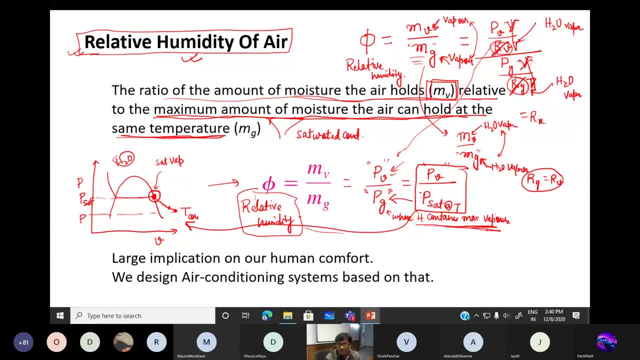 is written as the ratio of partial pressure of water vapor and the saturation pressure. Saturation pressure at that temperature. basically, Are you guys following it? Have you guys followed it? Yes, sir, good, Thank you. So it has a large implication on our human comfort. We design air conditioning system. 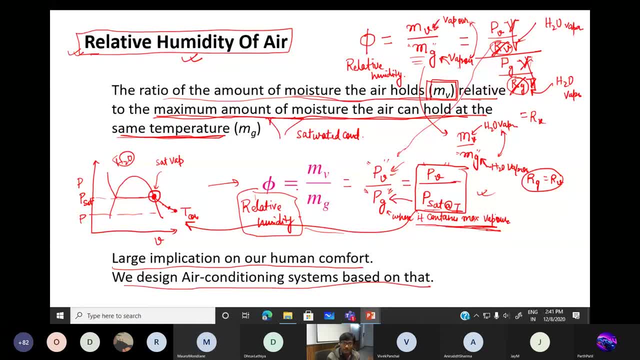 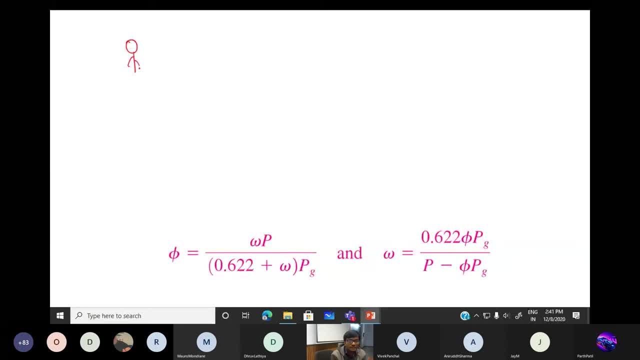 based on thatWhy. So, in general, in general, human needs 22 to 27 degree C. So you what your air conditioning does. it not only optimize your temperatures but also optimize your relative humidity. so, relative humidity, you may want things to be 40 to 60 percent actually, relative humidity. 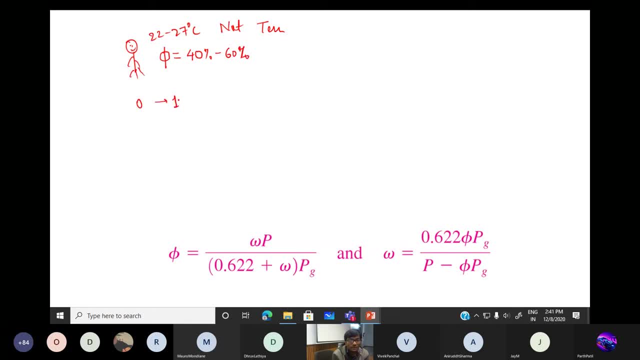 can go from 0 to 1. I mean 0 to 100 percent. so 100 percent, you will be sweating a lot, I am telling you. I mean everything will be. you will feel become waterly okay. so you want things to be for comfort thing. not only temperatures, but your relative humidity should also be. 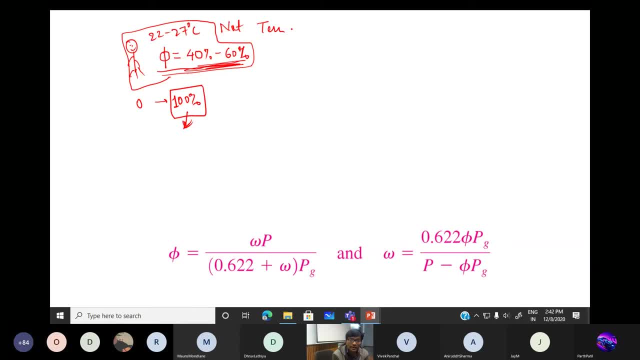 in certain range. okay so your air conditioning system, not only optimize your temperatures by throwing. by throwing I mean taking the heat from a sink and and, okay, you, you will be running some, some compressor and you are throwing the heat to source maybe lower temperature to higher temperature. okay so, not only you are doing. 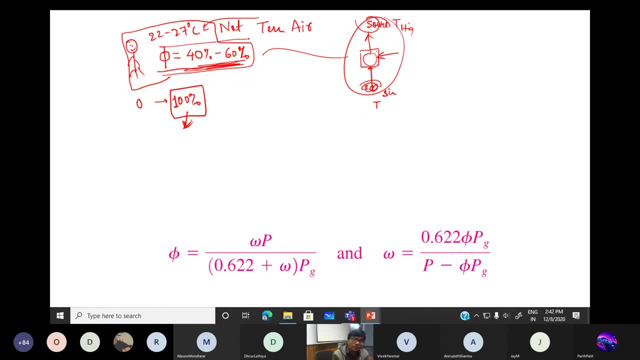 this, but you are also doing something like something to control your humidity as well. okay, how many of you guys know- know this- that air conditioning not only regulate your temperatures, but but also regulates your humidity level also, how many of you guys know this? none, yes, one, two, anybody. 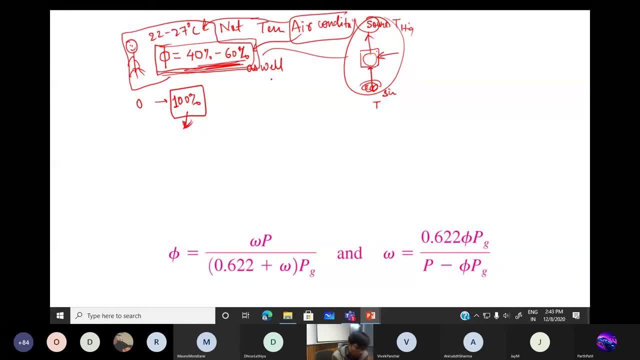 oh, you know, you knew this, okay, good, yes, sir. okay, air conditioners excrete water outside near the compressor. that is for humidity maintain. oh, exactly, exactly, thank you, who is this? okay, good, good, i think first time i'm talking to you. fine, so, yes, so we do. 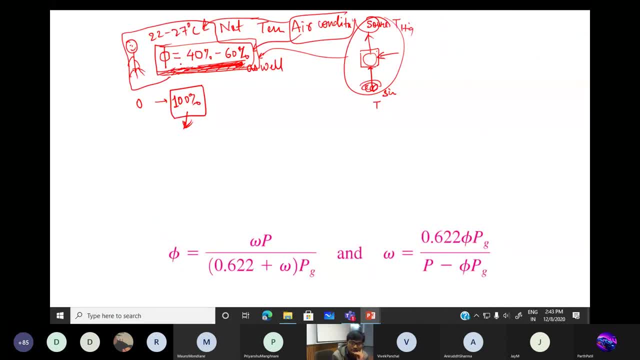 regulate uh, specific humidity, relative humidities and, in turn, specific humidity, because specific humidity, relative humidity and specific humidities are can be uh related. i mean, these are related, actually interrelated. you can get these expression by certain algebraic, so you, if you do some certain algebra, let's suppose this is. 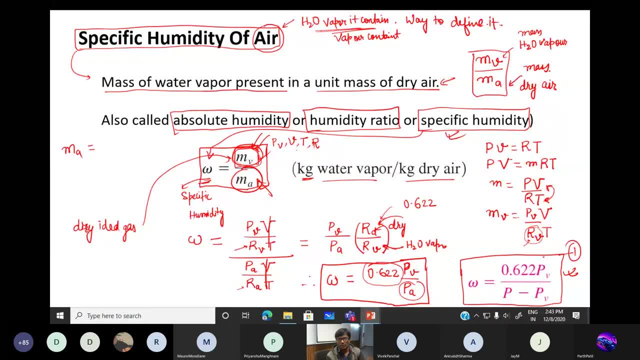 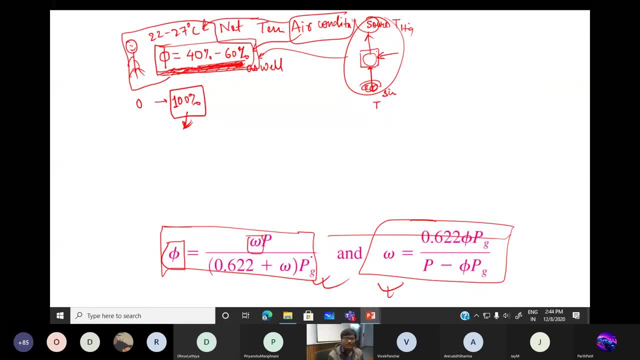 my equation one and this is your equation two. you can actually, uh, match things up and you can get this formula- and i will not go into the details of this algebra- but, yes, uh, in a way, you are actually regulating your specific and relative humidities, uh, with your air conditioning.